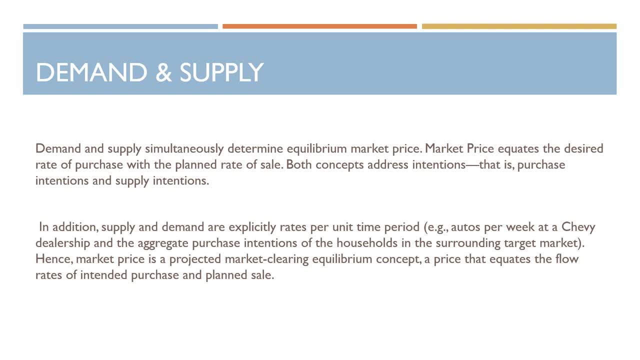 think about auto per week that produce at Chevy dealerships and the aggregate purchase and tensions of the households in the surrounding target markets. Market price is a projected market clearing equilibrium concept, which means a price that equates the flow rate of intended purchase and the planned sales by the firms. 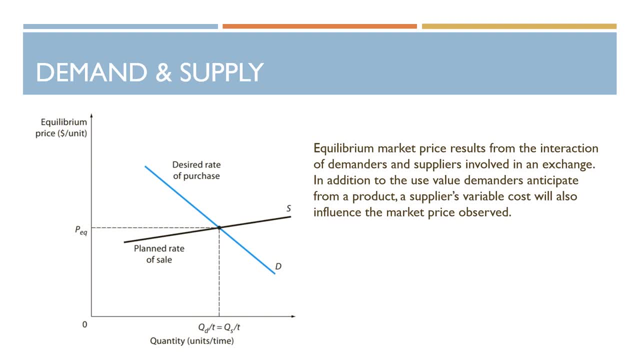 Many of you actually have seen this show on the market, this graph, before. looking at the supply and demand plots, we can easily find that equilibrium place where two lines are met At this equilibrium price. again, the concept is basically where the buyers and the sellers are committed to that. 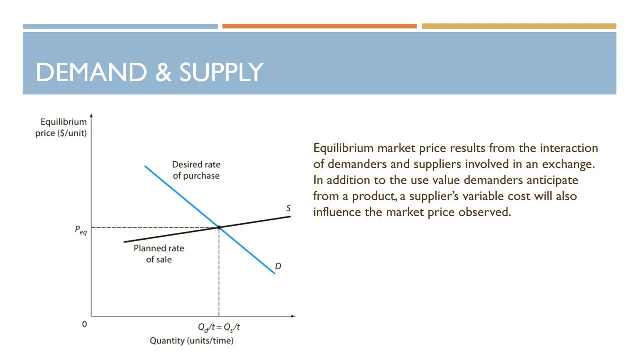 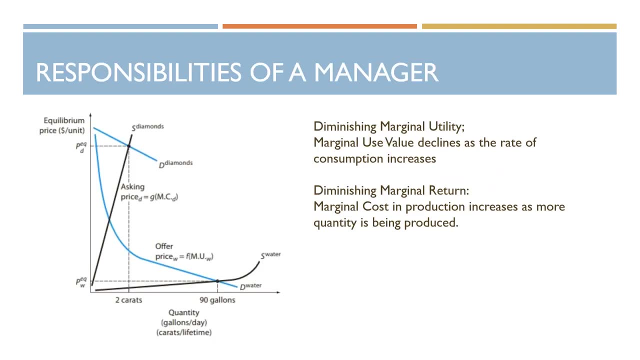 one price of the products in the market that actually drive the clearance of the inventory of the goods. However, there are many different contributions to this supply curve and demand curve that's shaping the curve differently. Some of the key concepts that you might want to: 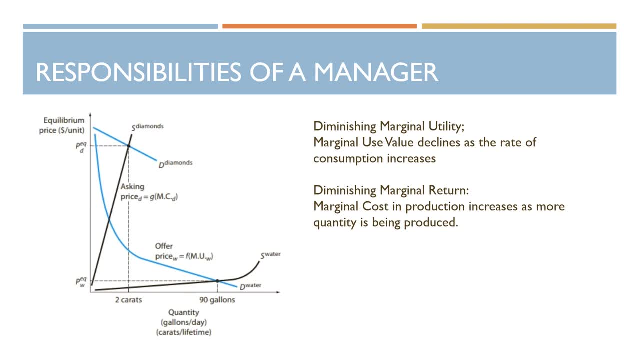 revisit are the following: Diminishing marginal utility. So the diminishing marginal utility is a concept that describes how consumers are, being it's ranking the product in the heads and trying to find a relative price that actually most reasonable for them to purchase the goods or service. When more of the same good is consumed, the lower the 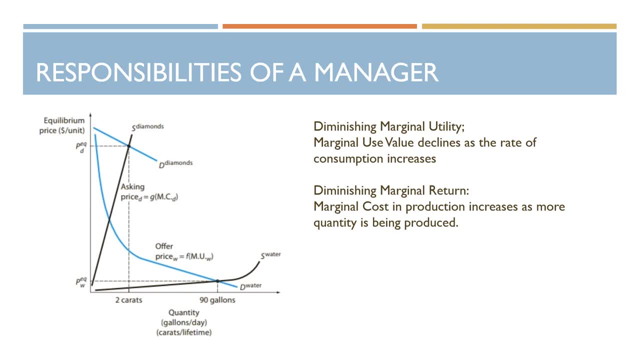 utilities that we think that we're gaining from that particular products And, as a result, the demand curve is actually downward shaping, mainly because, while everyone think that, well, eating the first burger it's great, it's worth $10.. Eating the second burger it's good, it's worth $8.. But the more 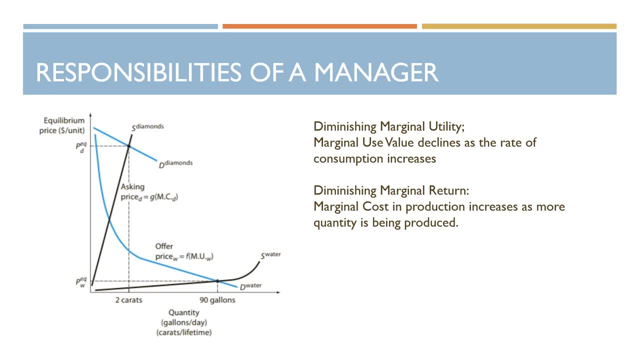 you eat at that particular point of time period, the lower additional utility you will get back- and that's where the diminishing part is coming from- And, as a result, the higher quantity of the goods that's being consumed in the market, the lower the price is required for people to purchase. 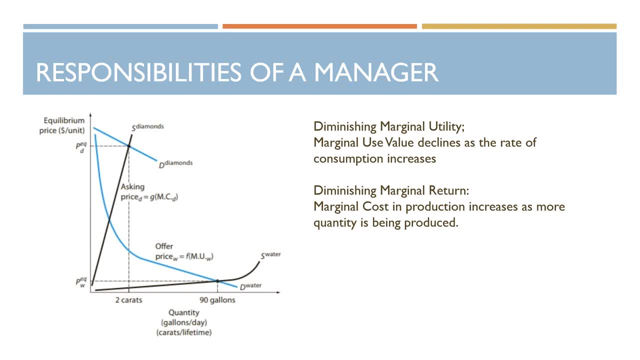 that amount of goods. Similarly, we have the concept of diminishing marginal returns, which is mainly described the cost side of the products. So the marginal cost in the production usually will be increasing. as many of you actually remember, there is a marginal cost curve study in Econ 101.. 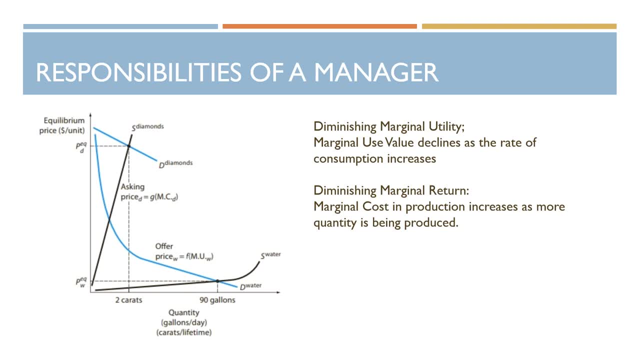 And the main reason for that is because, as more of the supply of goods increases, the more the cost of the goods increases. the more the cost of the goods increases, So the cost of the goods increases, the more the cost of the goods increases, So the 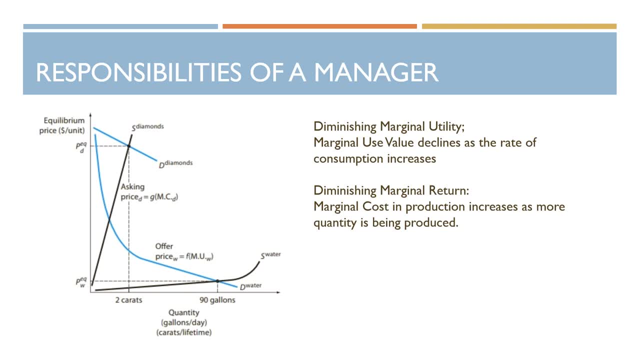 same product produced in a particular manufacturing setting, the higher the cost- additional cost, marginal cost will evolve And even though when we are trying to adjust the production inputs, for example, like labors or capital, but we are always bound by some fixed cost or fixed 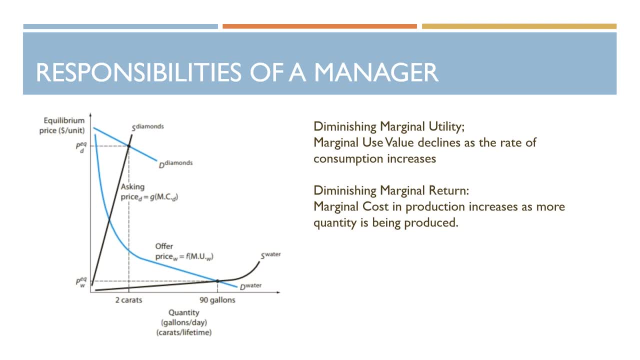 production factors, For example, like the size of the factories. we can continue to increase the number of people working in the factory, to drive more efficient work, divisions of work or specializations, to lower the cost, But at some point, when we have 500 people or 1000 people working in a very small, tiny factory space, 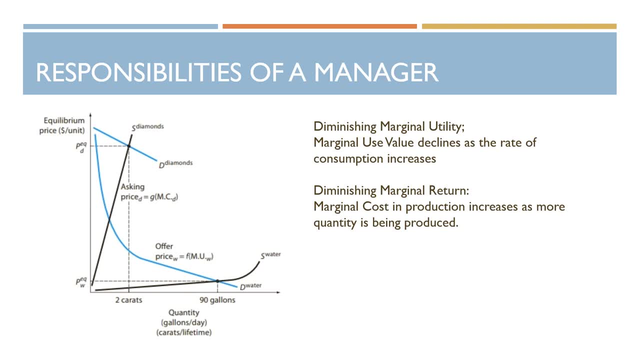 they are basically just packed in a similar in a small space that preventing more efficiency can come out from that. So these are the kinds of systems we have to work with as we come to being in a bear market with more scales because we want to have more capacity. 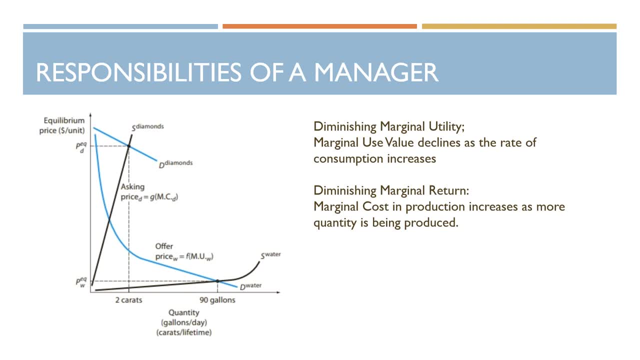 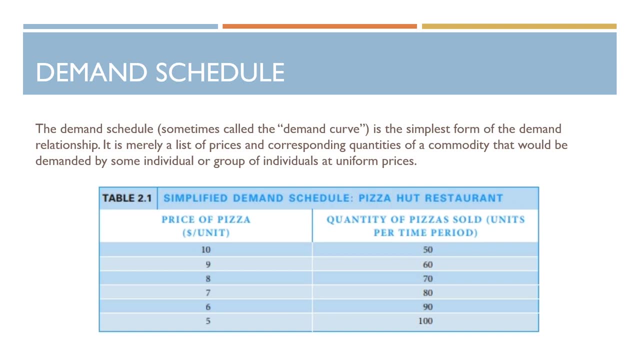 So in those- Those are the things thatев the supply, También en todos los estados territoriales- nos permit más capacidad de comida. So these marginal cost concepts, so this marginal cost concept, it's a fundamental idea that driving the supply curve, There are many things that we use to describe the supply and demand in the market and one of the particular type on the market. 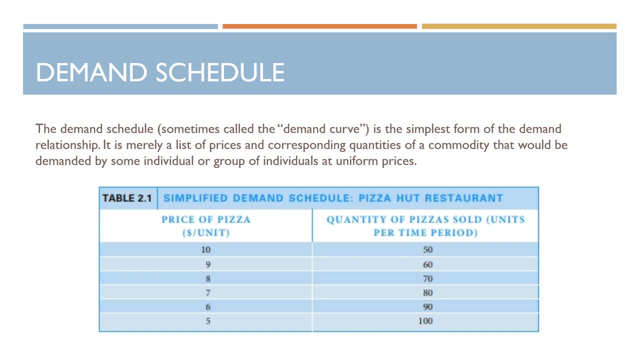 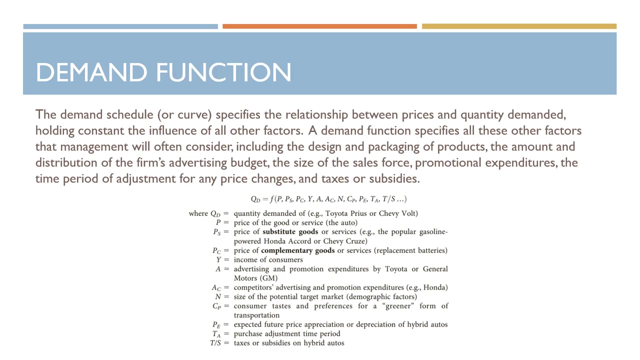 Maybe the tools that we use. It's called the demand schedules. So the demand schedule It's basically the tablet To indicate demand in demand, shows you the quantity being demanded in the market versus the price at that particular quantity demanded situations. again back to econ 101. there are many attributes to the demand functions or 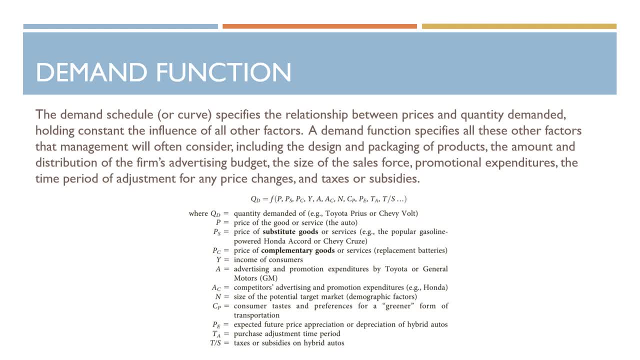 driving the demand right in the market. when we say driving the demand or maybe shifting the demand curve, or maybe changing the demand of a good, we are literally thinking of. the demand curve is shifting either left or the right, so for example, the price of the good itself, it's not a shifting. 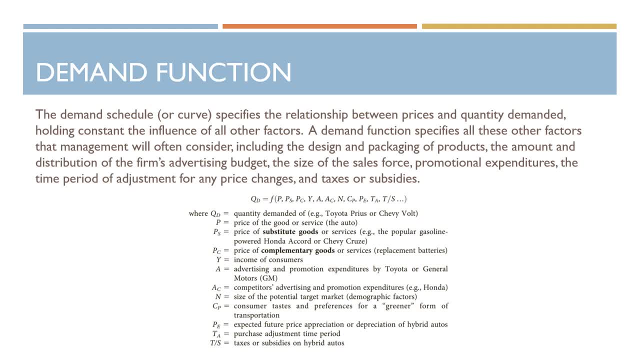 factor of the demand, so it doesn't shift the curve. the price of the good itself basically affects the price of the demand. quantity demands of the goods. however, the price of the substitute goods or complement goods, they are the shifting factors of the demand. the income of the populations in the markets also is a 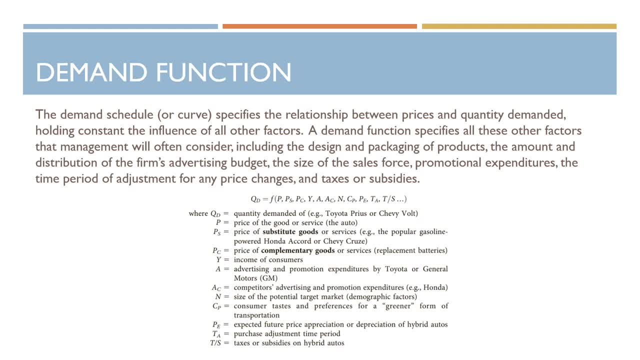 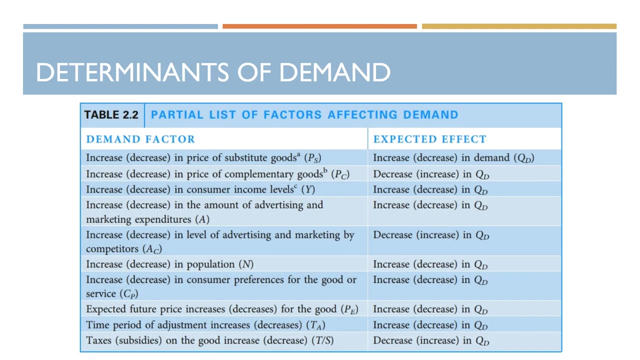 shifting factor. the size of the markets, how many people are exist in the market, taste and preferences, the expected future price of the goods change- all of this are basically contributes to the shift of the demand curve, or sometimes we call this the change in demand. here's a list of the determinants of demands. again, those are the fundamental factors that 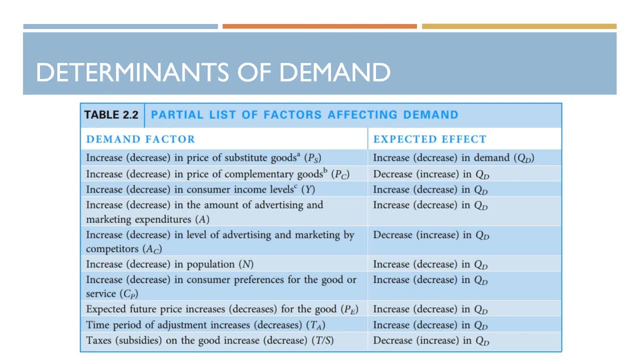 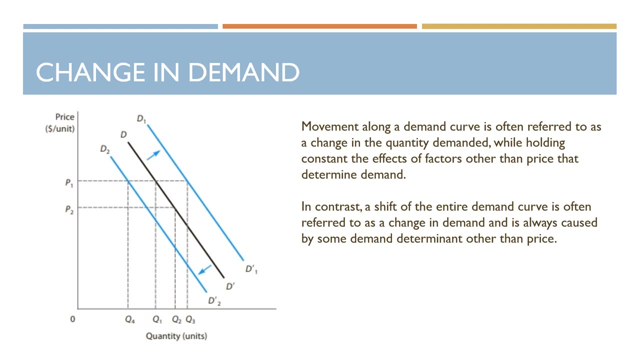 we study as an economist to find out why something is getting more expensive or being demanded in the markets, as comparing to different time periods. so the concept here again shifting the demand curve. it's not associated with the vertical attitude change but it's more fundamentally referring to the left or right horizontal shifts of the curve. 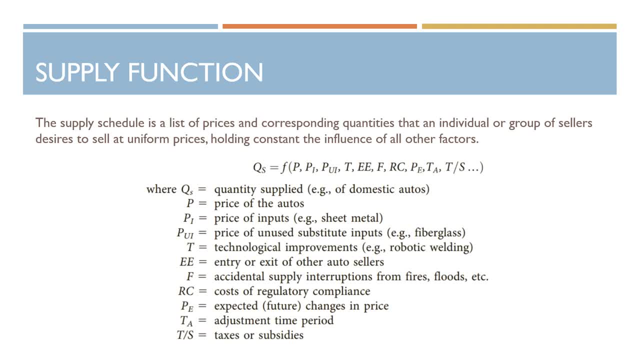 on the other hand, supply also have the similar factors that actually changing the supply of goods. for example, the price of the production inputs, the price of the unused substitute inputs, the technological improvements, the number of sellers exist in the market, the costs for for complying some sort of regulatory compliances, tax also expected change in prices in the markets. 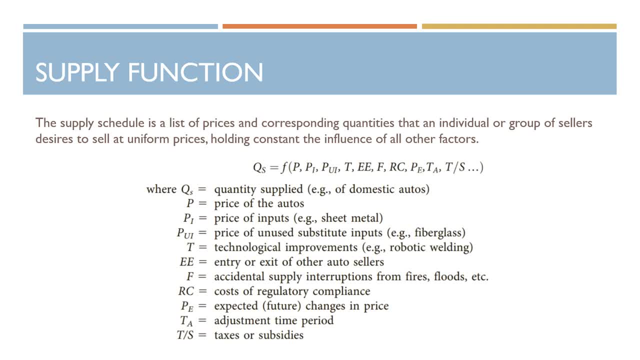 in the future. so all of this are basically what we call the determinants of supply or the shifters of the supply curve. so the demand curve is a model of supply and demand curve and that's what we call the. So again, the concept here is the supply curve will be shifting either left or right based on the change of these factors in the market. 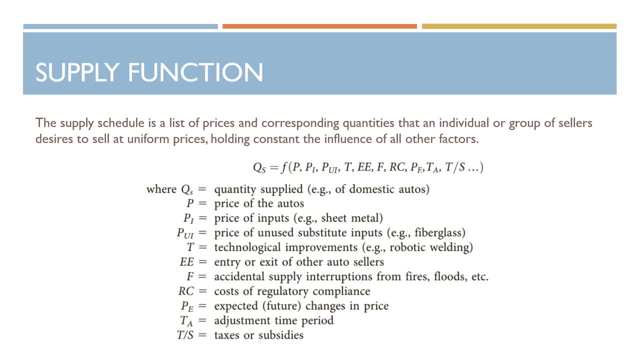 But keep in mind the price of the product itself. it's never a shifting factor of either a demand or supply of the goods. The price of the product. it's going to affect the quantity demanded of the goods or the quantity supplied of the goods in the market. 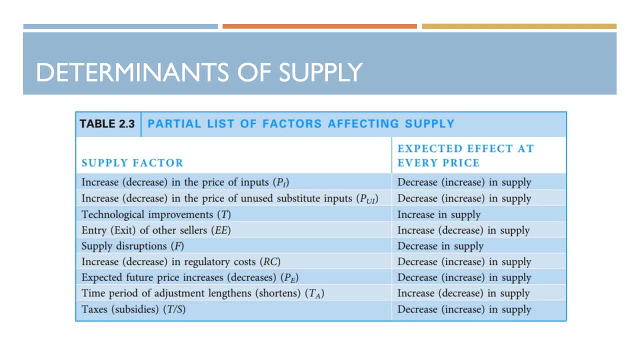 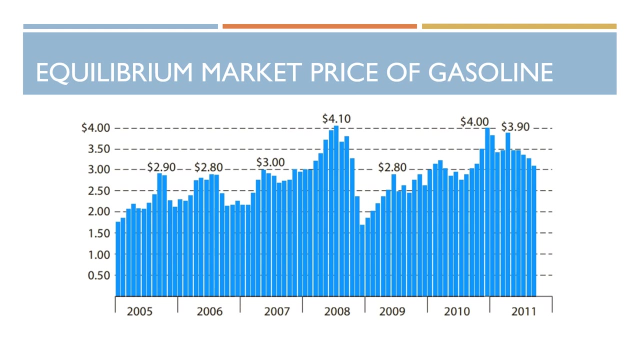 Again, there's a table of a list of the supply factors that's shifting the supply curve either left or right. Here's an example of the price of gasoline from the year of 2005 to 2011.. So at every single point of time, as you can see, there is a price that is committed. 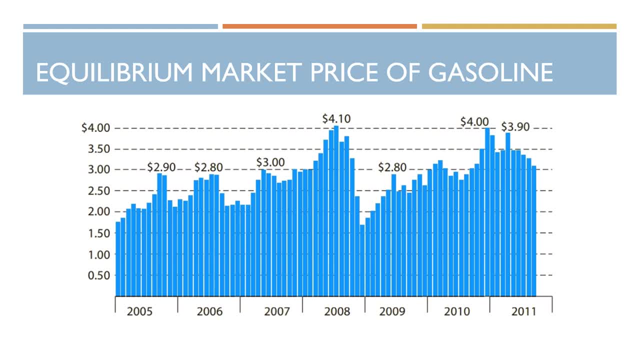 It's a price that is committed In that particular month in this case. so we have 12 months in a year and each bar represents the price of gasoline in that particular month. So you can literally tell that at certain time of the year the price of gasoline will be higher as comparing to the other month. 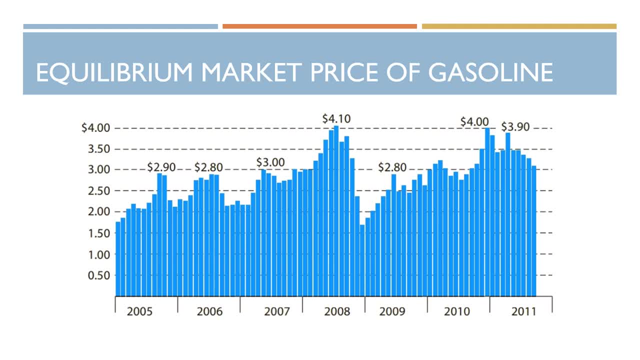 And obviously the intuitive reasoning here is that in some point of the years people will have to consume More electricity, And when they usually do- as you can observe from the graph- either the summertime or the wintertime right. 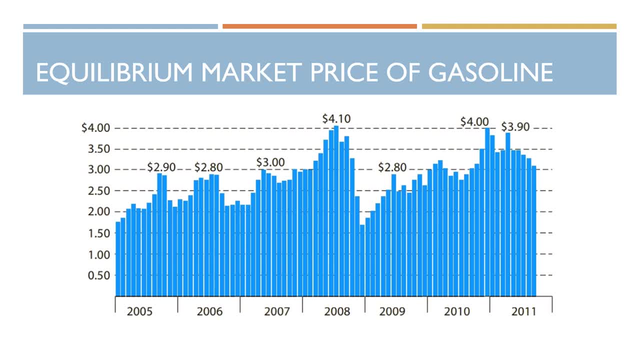 So either people are turning on their AC or maybe the heater- Those are the basically the most demanded periods of gasoline- or maybe traveling right in the summer, where the gasoline prices will be demanded the most And, as a result, the price of, Or the equilibrium price in this case. 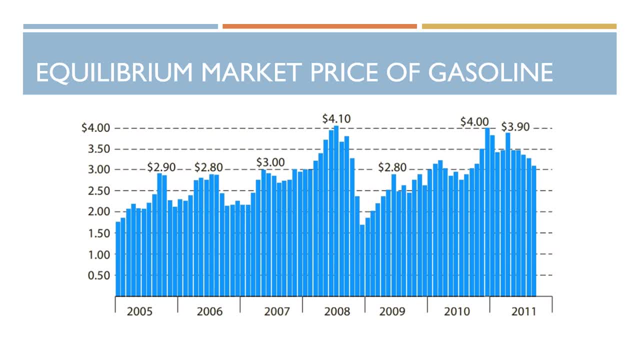 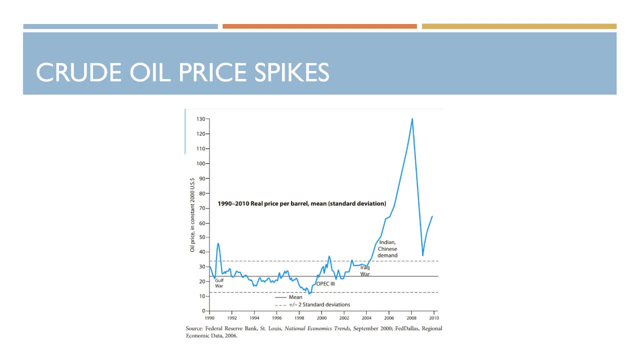 Will be higher in those periods. So what were the other factors that the state was careful about? So New Zealand eggs being silent on what was actually happening, but also the difference in students saying that M160 does not count for the of or four years. 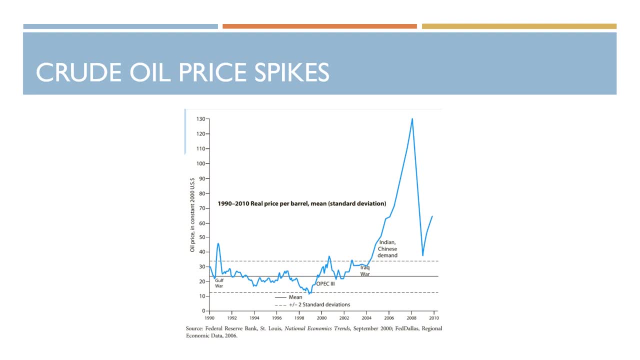 Well, of course there are increasing and it's always negative. But if you take into account some of the changes in the taxes that the state and M terra crois To get going, then it's very unlikely that that earnings level is going to be good or, you know, might change. Does that tell that youre the right nessa? What is that? Yeah, Yeah. So if I look at Joined JOE E, I think you know I loved listening toieng sam and Roe Dahl- the lad- from concluding theirоты me. 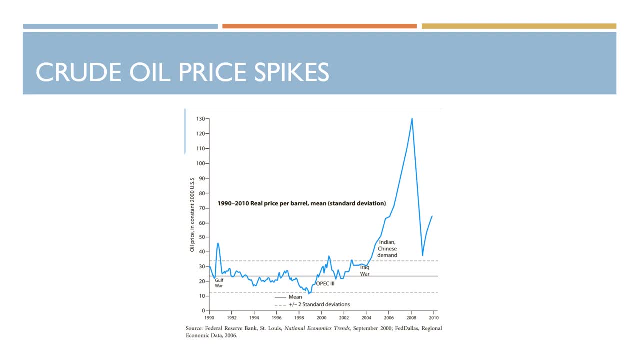 So you're talking about things that work just fine. it didn't work out right, And mainly because of the Iraq War after that, where the supply of crude oil imported to the United States has- or maybe not just the United States, but the worldwide has- changed dramatically. 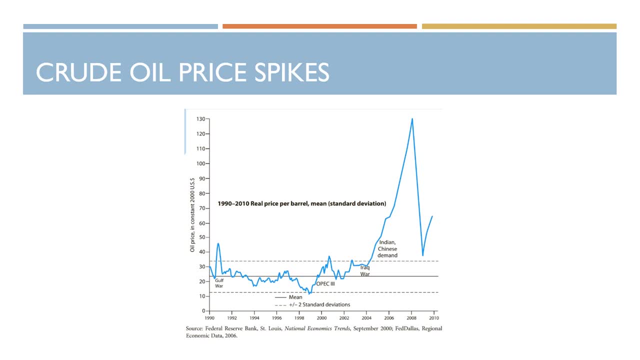 So, because of the change of supply, in this case the supply curve shifting dramatically to the left and affecting the oil prices or the crude oil prices in the international markets to be at a higher level, And you are seeing this equilibrium price in the year of 2004 to 2010 has jumped dramatically to from about 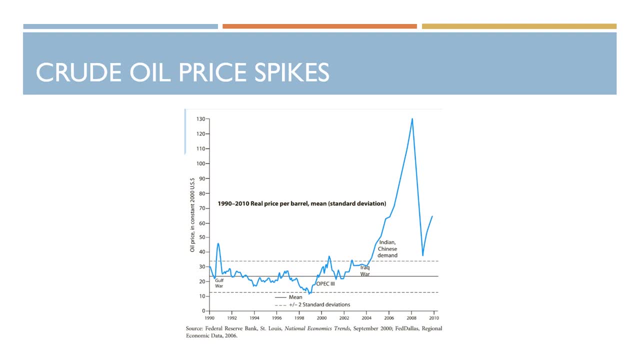 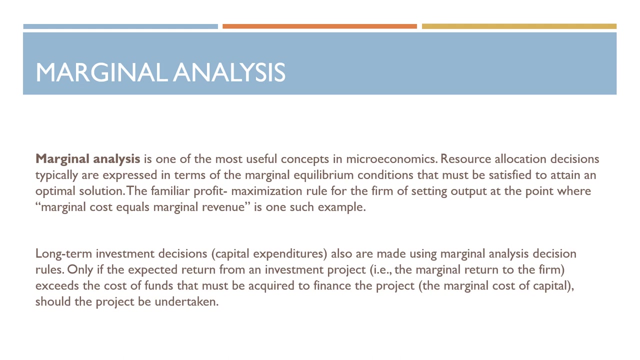 $40 or maybe $35, all the way up to $130 in the year of 2008,, and then come back down to the $40 range in 2010.. So the reason why we are talking about supply and demand is because we want to always keep in mind every business decisions are based on the fact that whether there is a market to do business, 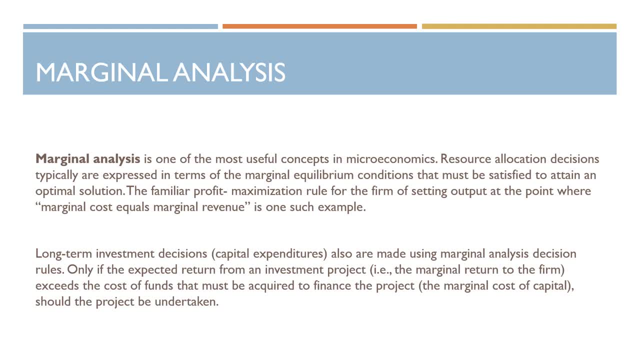 And the markets, it's always represented by either the supply side or the demand side, right. So there's never one market where supply actually represents the whole market or the demand represents the whole market. There are some cases that we will study later to talk about the monopoly case, which is one supplier supplying the goods to the whole market. 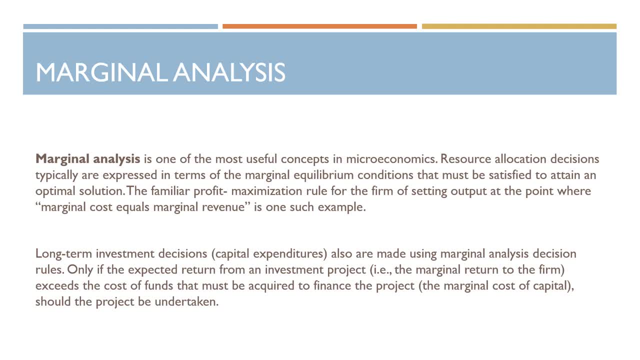 But again, if there is no consumer, even with the monopoly firms, there is no market to be defined. Okay, So, talking about business decisions, most of the time people are confused about how decision is being made or at what magnitudes it should be made. 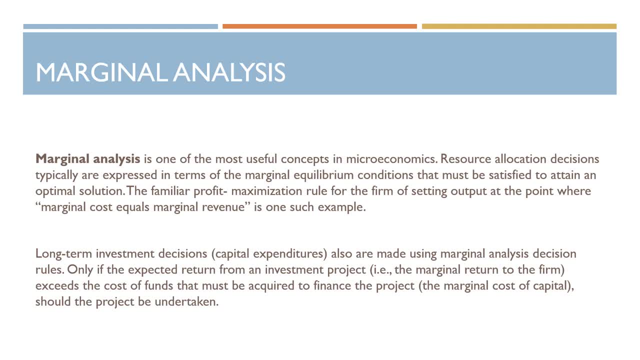 So in economics we actually define economic decisions or business decisions at a marginals. So we don't think most of these business decisions is made by just saying either we do it or not, or we are all in from our resources to achieve one project or we put all the resources to another project. 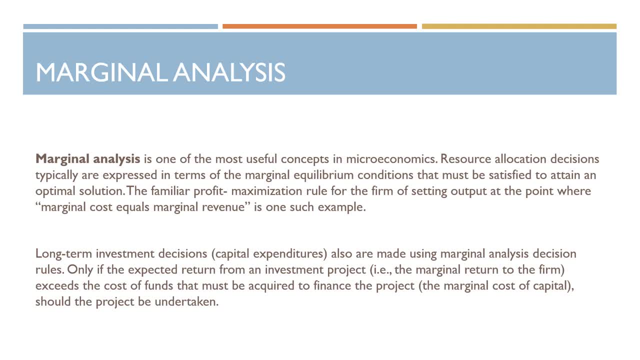 But we are mostly thinking about allocations of the resources and the marginals, right? So how much we should be spending on developing a product versus how much resources we should spend on marketing, how much resources we should spend on managing our finance- Right. 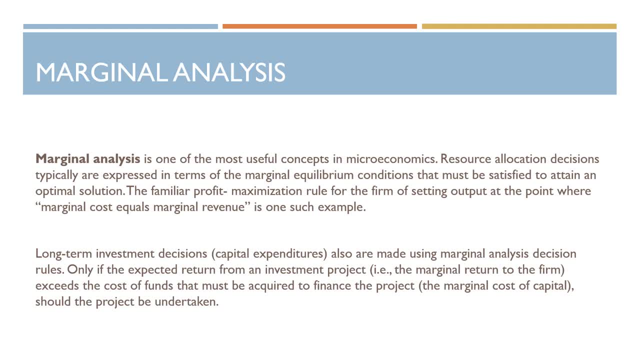 the company. so all of this are basically what we call a marginal analysis: what resources should be used. it's based on what the marginal benefits we can get out from those resources and how much does it cost us relatively to other factors in our in a business decisions. so the long-term investment. 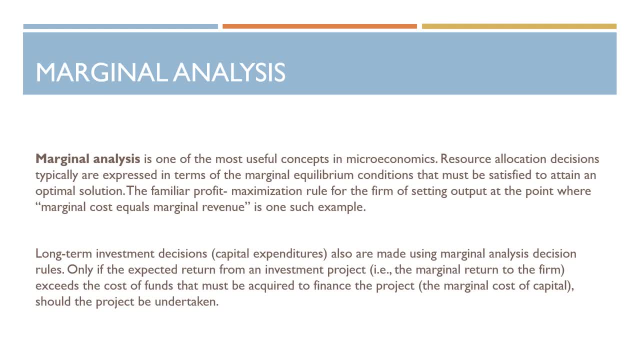 decisions or the capital expenditure, also made by using the marginal analysis decision rules, where the marginal benefits is equal to marginal cost. this is the golden rule of thumb, where the profit can be maximized, but only if the expected return from the investment project actually exceeds the cost of the funds. then well, the project will be considered to be. 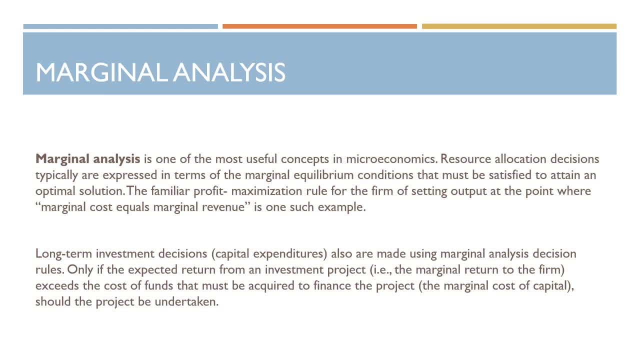 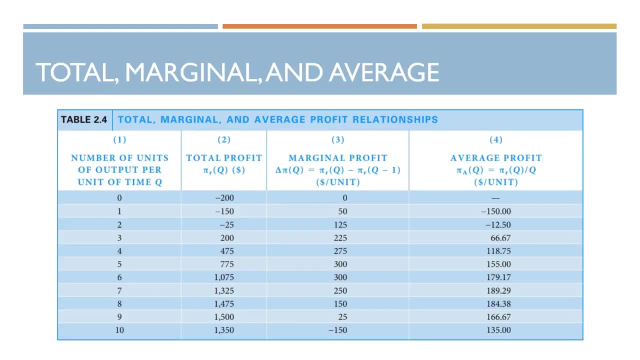 profitable. otherwise the project should be under ticket right. so talking about marginals, again going back to econ 101, most of you already have a concept about marginal cost, marginal revenues and, of course, marginal benefits, which is marginal profits of a firm. but to have a little bit better idea about how those 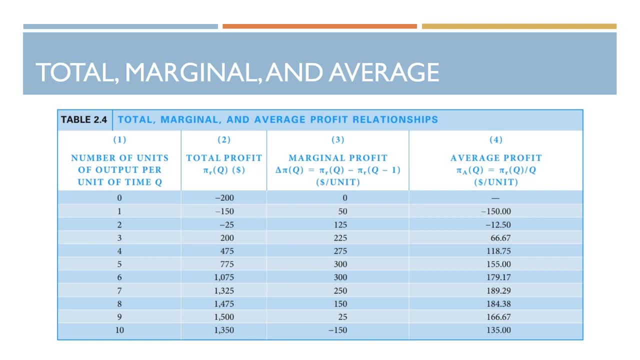 uh number is associated to each other. you can look at this particular example here. table here actually represent four columns. the first column represent the number of units of outputs that the firm produced or sell in the market. the second column is the total profits earned from that particular unit cell in the market and the third columns represent the marginal profits. how much? 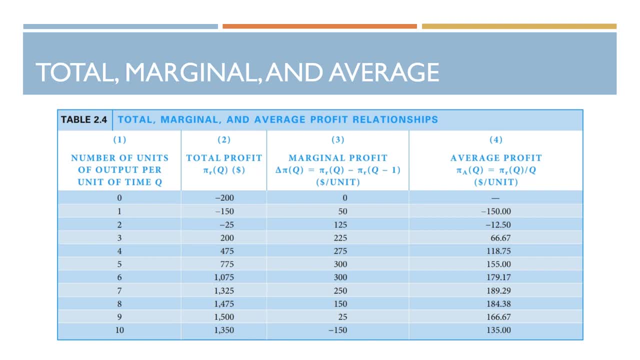 additional profits we can get from that number. so to have a little bit better idea about how the We can get out from selling one more unit of the product or service. And the last columns there represent the average profit, which is the total number of profits divided by the total number of outputs sold by the firm. 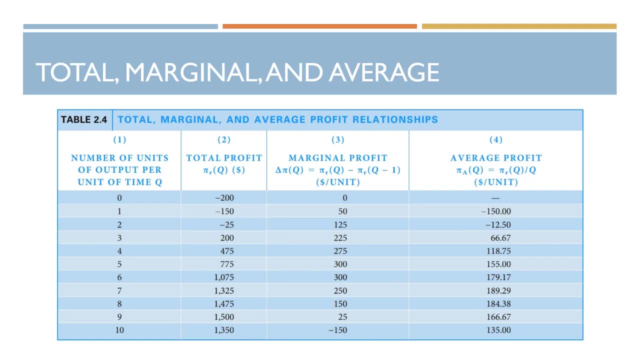 Well, in this case you can totally see how the total profits most of the time does not speak out the true story of the firm right? So when you are making decisions you look at: oh, the business will lose $200, $150 or $25 when the firm selling zero unit, one unit or two units in the 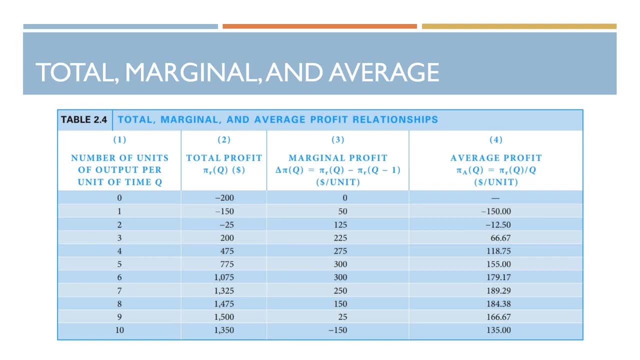 market. but that's not the story. that is good for your decision-making, because How you want to determine what is the maximum amounts of output to produce to maximize profits, You probably care much about The marginal profit in this case. well, selling one more, how much? 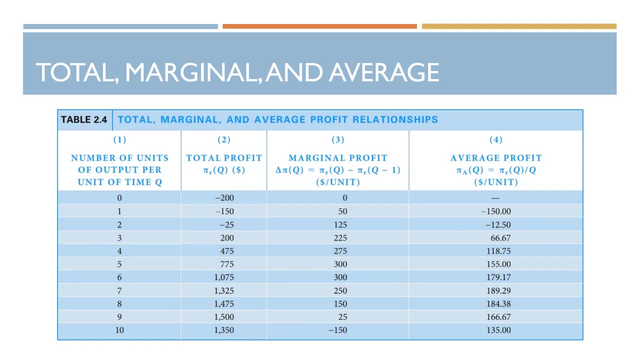 additional profits the firm can earn. And that, basically, is the fundamental idea Why this table here. it's so valuable because, if you look at it, the at the beginning, it doesn't seem like the firm is getting much out of the um, uh, the. 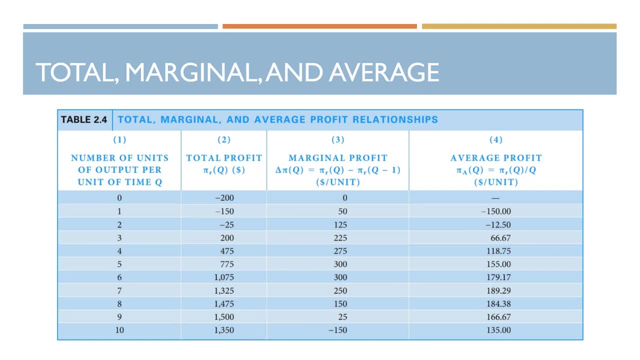 productions. particularly if we look at zero, one, two, three, uh uh units of productions, the firm actually getting negative profits. So does that mean the firm should never produce the goods? And the answer, of course, is no right. 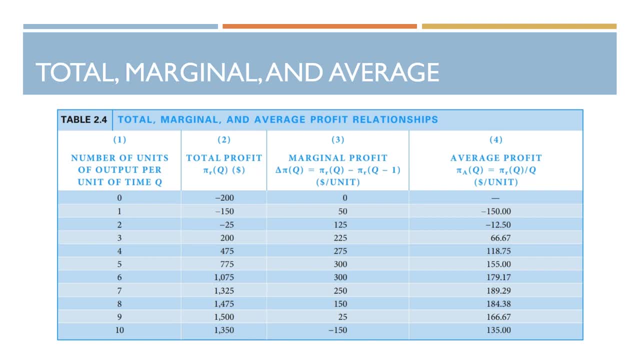 So we want to actually look at the marginal profits. If the firm continue to produce more, how much additional they can get in returns. And in this case the firm can continue to produce this good until unit number nine where the firms actually earn $25 additionals more from producing that units. 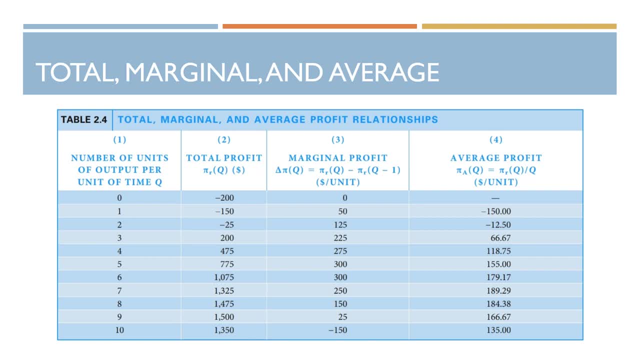 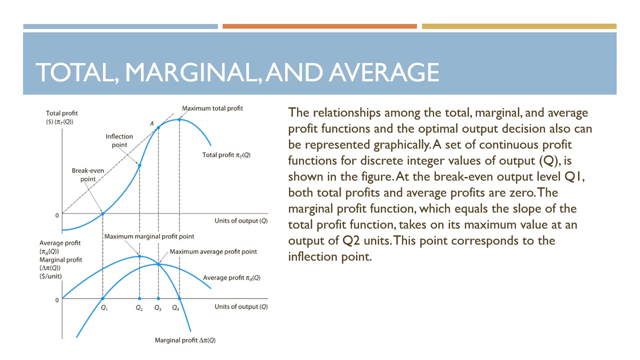 in the market, But the firm will never consider producing the 10 units, And the reason is because producing that 10 units will start with using the total profits on the firm earns in the market, which is counterintuitive. There are some visualizations in the econ one-on-one textbook that might 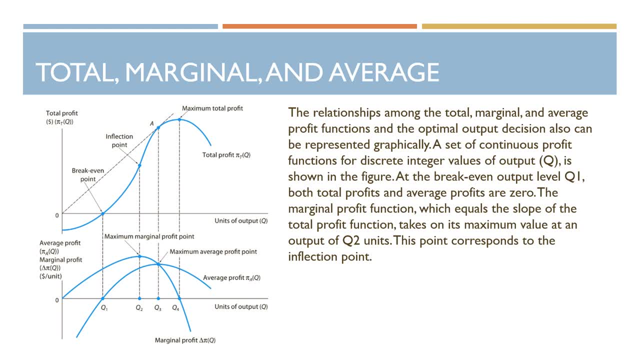 actually help you to understand the profit maximization rule or maybe the Optimizations uh uh concept here. Um, but the general idea is, if we are running a business and to seek for the uh profit maximize uh- points of outputs of the company, we most likely will care about. 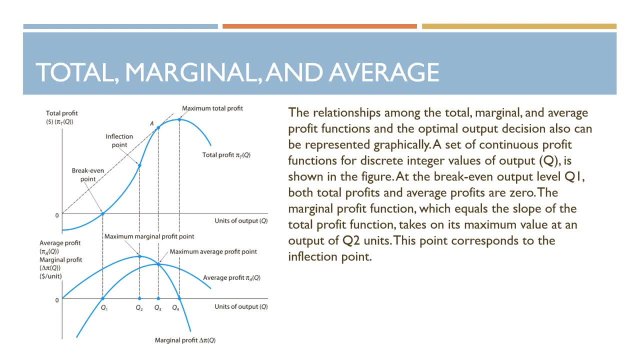 the marginal costs and the marginal revenues, uh, for selling the goods. Um and again, just back to the golden rules. The golden rules here basically suggest: if you have a situation where the marginal cost is almost equals to marginal benefits, right. 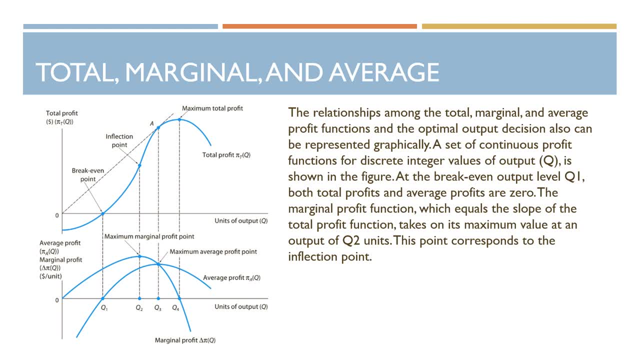 Which is the marginal revenues. Um, and that could be the break even, uh, levels of outputs that you want to produce as a firm to maximize the profits. Otherwise, producing anything more, the costs, or the additional costs, will be higher than the additional revenue and it. 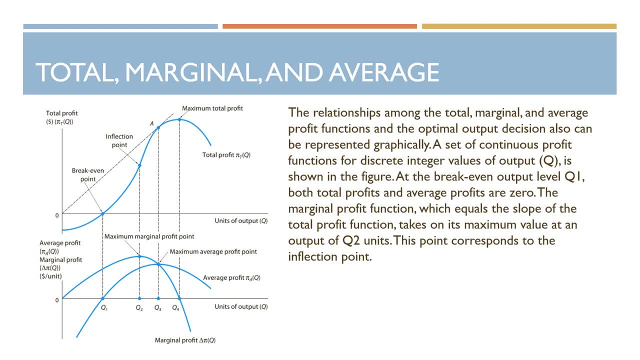 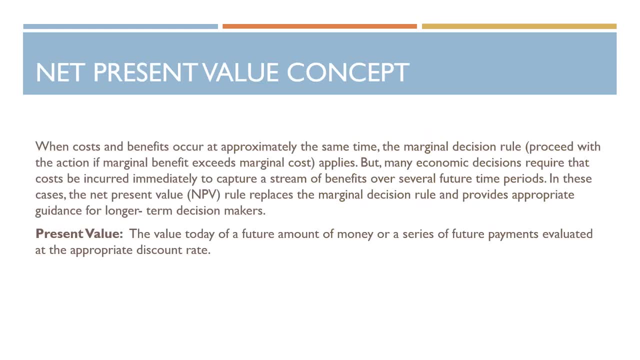 actually makes the company earning less profits in uh generals. Well, another very important things to note is that most of the time when company investing the money into projects, um, for example, like uh starting a new production lines or develop a new products, or maybe putting uh human resources to develop a software, uh for service. 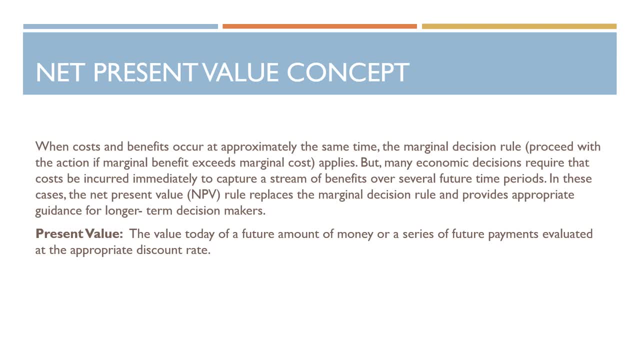 Uh base subscriptions um. all of this involved times to develop, produce and plan um, and the revenues might not comes into your company immediately after you have determined uh to go with the projects as a results, when uh many managers uh they are making their uh economic decisions for the business. 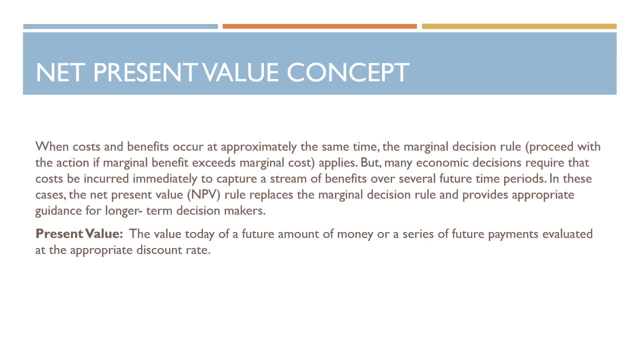 They usually don't consider the Um, what the revenues looks like right now or what they plans to earn in the next three months or three years, because, well, those values are not comparable to today's values of a dollar Um. so the idea here is um instead of just looking at a project and assuming that, well, one year later, when we start selling the goods, we are going to get $1 million back in revenues. 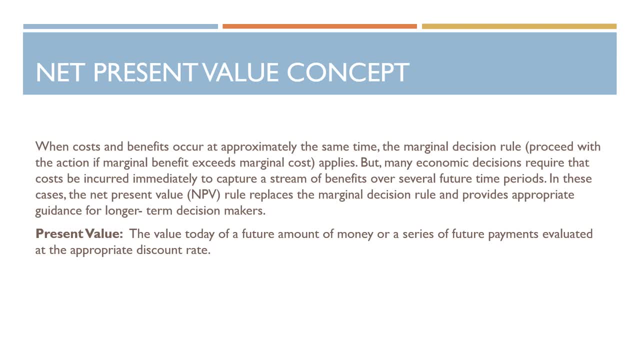 Uh, but we want to ask the questions: how much of that $1 million in a year later will worth in the present values. How much does it work nowadays? Um, and because of the depreciations of dollar or inflation in general, um, the dollar earned one year later definitely will have less purchasing power comparing to today's $1 million. and to calculate that we can actually apply, 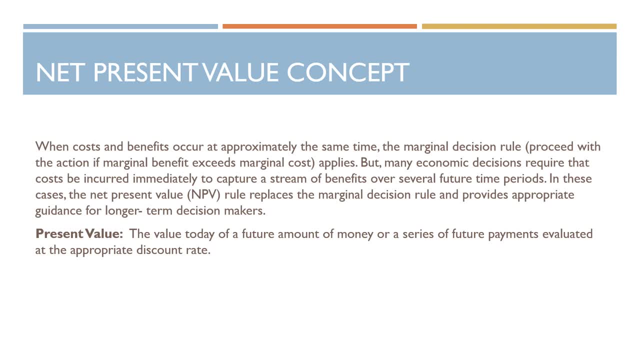 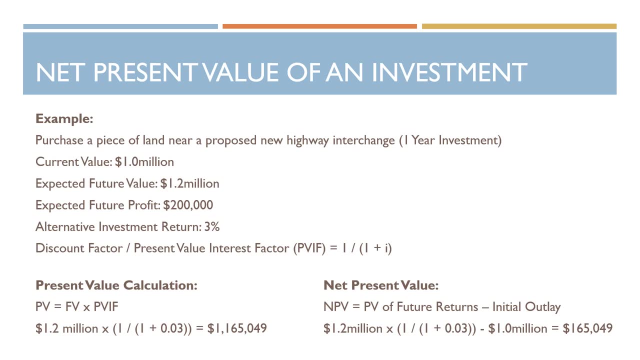 Some very simple mathematical process to calculate the present values of a um Pacific projects. So, given the example here, let's suppose we have a piece of land near a proposed new highway interchange. So it's a one year investment, The current value of the project it's $1 million and we're expecting the future value to uh return $1.2 million in this project. 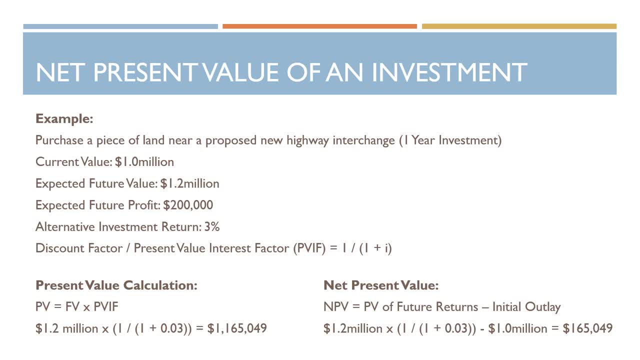 So that means the expected future profits will be $200,000. sounds pretty good, and there is a alternative: investments that actually provide us with 3% returns- uh, a year later as well. So let's say: well, there are two options here, and as a manager, I have to make a decisions. 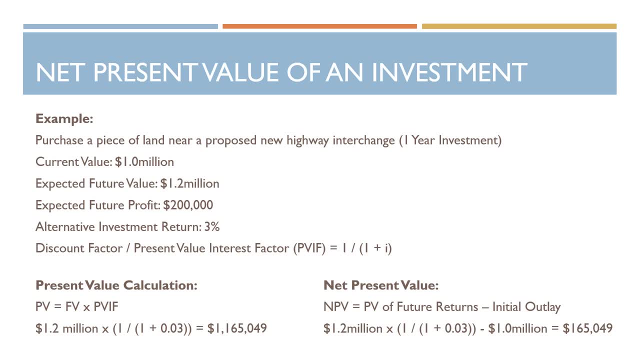 Should we invest our $1 million into this highway project or should we actually fund this? alternative investments returns. The way how we are going to determine um this can use uh the following equations: So in this case we are considering there is a discount factors um in this uh one year time period. 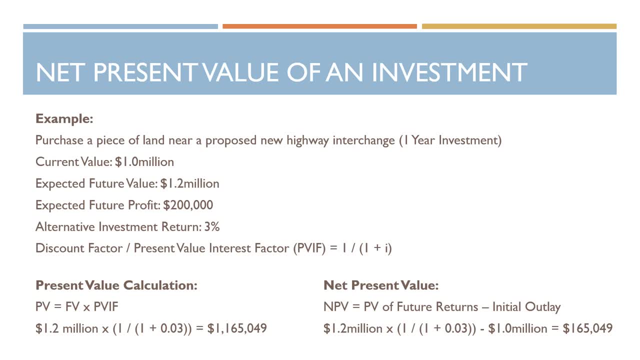 So this discount factor basically means that, well, one year later the money will, with no risk, to increase by 3% if we invest it into the alternative investments. However, because we want to compare the two head-to-heads, let's suppose money is going to grow 3% or maybe 3% later. discounted back in one year, which is today, it will be less than 3% of worth. 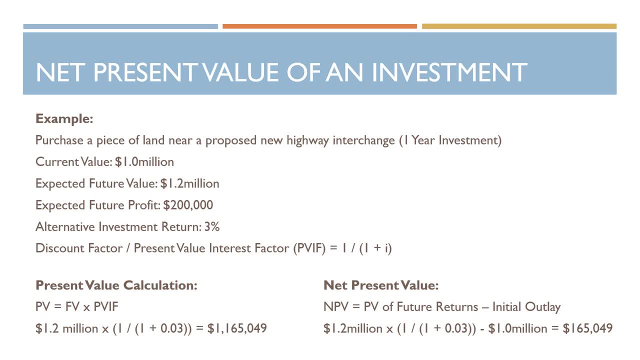 In this case we can actually use uh, the present value calculations, which is present values equals to the future values times, the future value interest factor And in this case, the future value in uh um uh interest factor is using the simple calculation, one divided by one plus 0.03.. 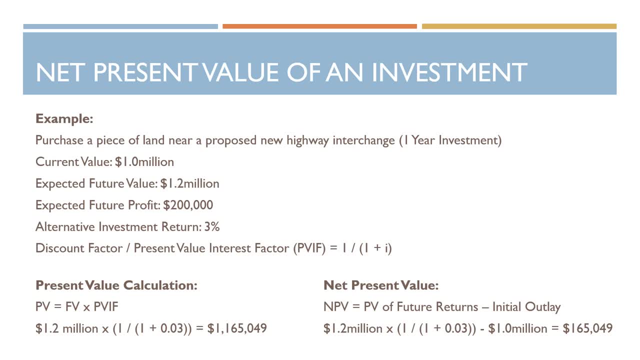 And using 1.2 million, which is the expected future value earned from the highway projects, times the interest factor and we will get $1.165 million, And this is basically the present values of the project. Consider if we are going to see money to grow 3% one year later, right into the future. 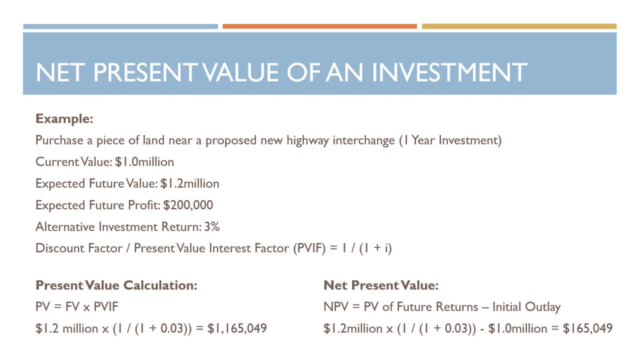 You can also do the calculation in the reverse way. to basically ask the question: what would be the net present values? Um, if we are going to fund this uh project and getting the money, uh, one year later, how much that $200,000 will worth? uh, that, um, uh, uh, uh, uh, uh for today. 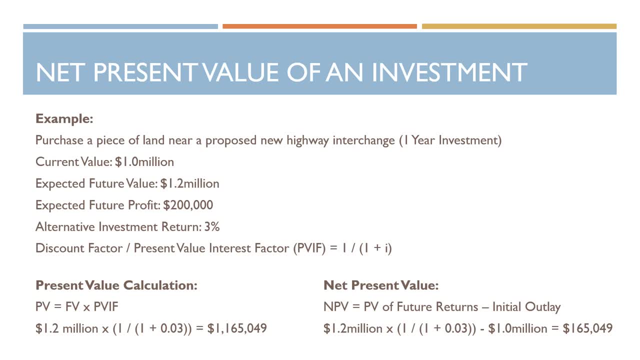 So in this case, we're using the $1.2 million, which is the present values, uh of future returns, uh times uh one over one plus 0.03.. Um, and then we use this uh uh present value of future returns minus what we initially uh invested to this project, which is $1 million. 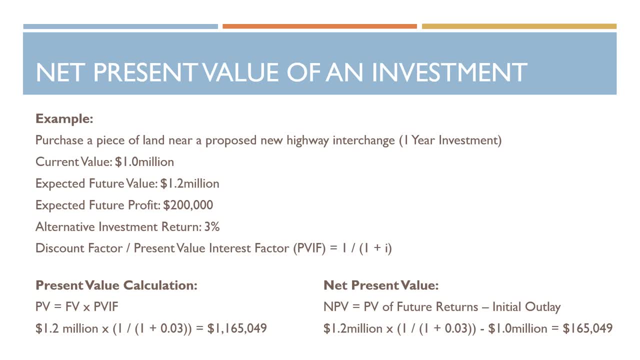 And in this case, uh, the 1.165 million minus 1 million, we have Uh now $165,000, and that's basically the net present values. return from this projects. uh, one year later, as of today's purchasing power- because assuming the money is going to grow- 3% for whatever uh uh situation that could be. 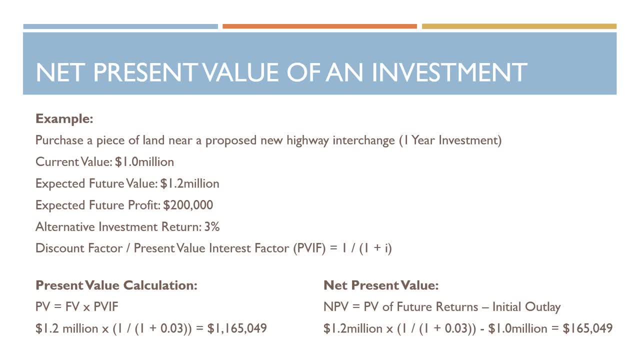 So, using this example, you can, you can simply think about if we are, We are adjusting with inflation, Right? Uh, one year later, instead of using the 3% as an investment returns, we can actually replace that number with any inflation figures. uh, in the current state of the economy, 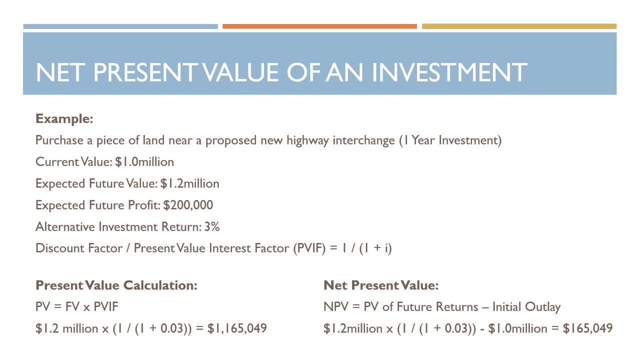 So, for example, if the current state of economy has an inflation of 5%, then you can replace the 3% with the 5% and assuming money is going to depreciate 3% a year later, So how much that money actually? 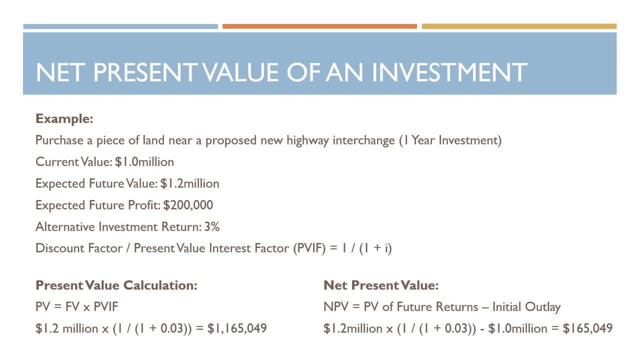 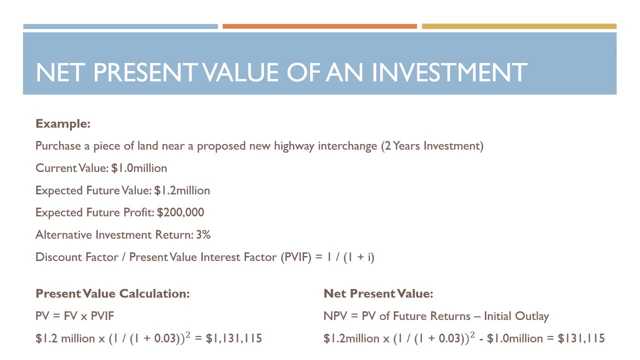 Actually worth uh for today's if we are investing into this projects. Well, another example here, basically just for um, the comparison purpose when the project goes into two years, uh, and how we are going to calculate the compounds uh valuations, uh, by taking the square of that present value interest factor in our calculations. 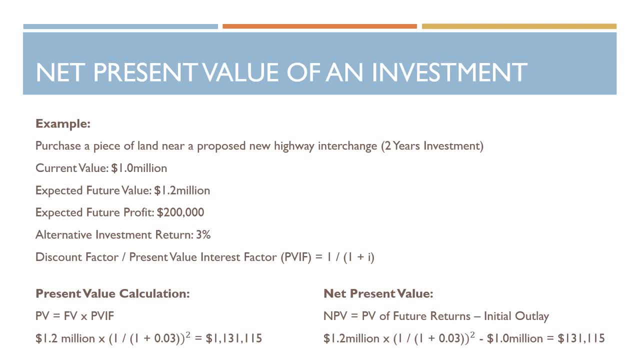 And, of course, you can continue to ask the question: what about the year goes, uh, what about the project goes into three years or four years or even five years, And, uh, the things that you need to do, it's basically compound the interest, uh factors, by the power of the terms. 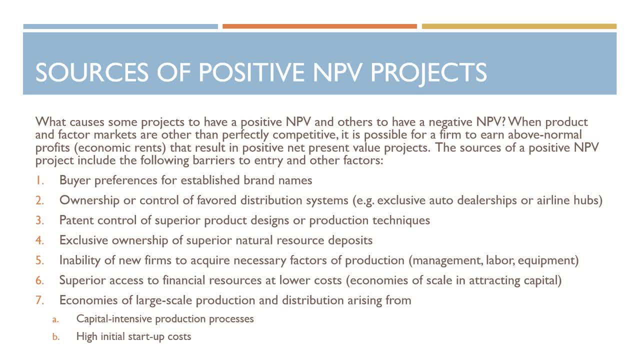 So what costs some projects to have positive? uh net present values and uh what causes some of them to be negative? So when the products and the factor markets are often perfectly competitive, it's it is possible for the firm to earn above normal profits, or what we call the economic rents. 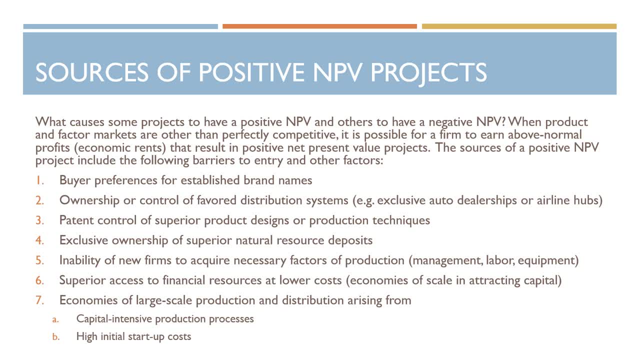 Um as a result in positive net present value projects. the source of the positive net present value project includes the following barriers to entry or maybe other factors in the markets. For example, number one: we have the buyer preferences. change uh or established a brand name. 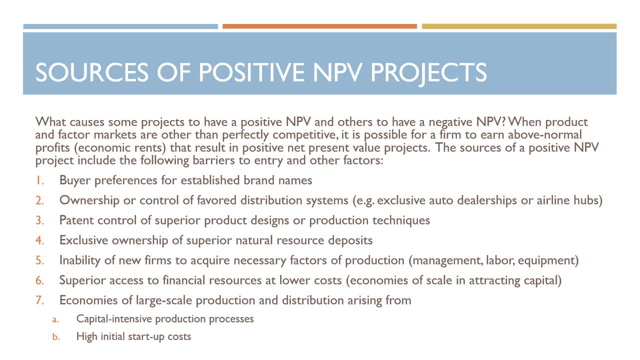 So that people think the brand is actually well qualified, uh uh, has a good quality, or maybe it has a good reputations, It has a a well-developed cultures, um uh like environmental, established. um, people actually prefer buying more of this brand. 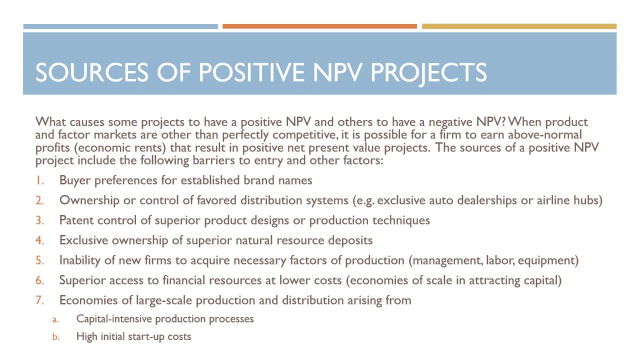 Then it makes it easier for the firm to earn uh a positive uh NPV uh number two ownerships uh control of favor distribution system, right? So if you're taking a control of a distribution System uh, for example, you exclusively uh have the ownerships of the auto dealerships uh, or maybe the airline hubs uh that dominates uh particular locations that you, you're basically earning all the all the businesses within the geographical locations. 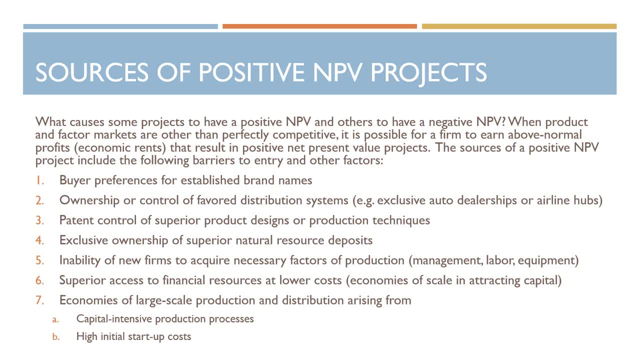 Uh, in those cases again, it makes it easier for a positive uh net present value returns, Pattern controls, um, or maybe uh any specific uh uh production Techniques or technologies, designs, uh that it's not easy to be replicates uh exclusive ownerships of the super superior natural resources. 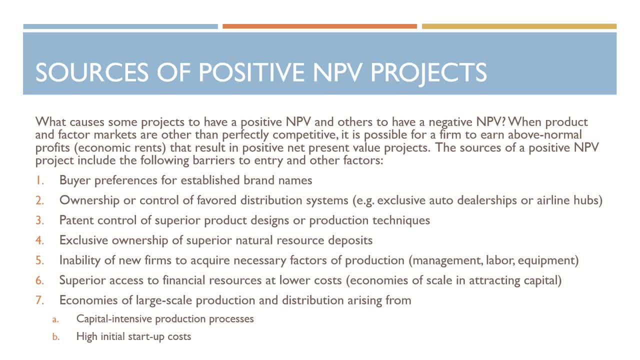 Uh, for example, some company owns a mine of code, then obviously this company might have a better hands to to uh mark up their prices in the markets. uh, inability of new firms to acquire necessary factors of productions, for example like management's labor equipment. 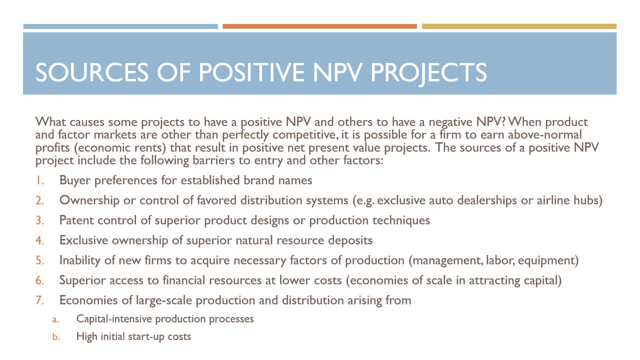 Um superior Access to financials, uh resources at a lower cost. So uh company that taking economy of scales to lower the cost attract capitals. Uh, those are the uh ones that again uh most likely to have a positive uh net present values. um taking economy of scales in production distributions arising from, for example, capital intensive production process or high initial startup costs. 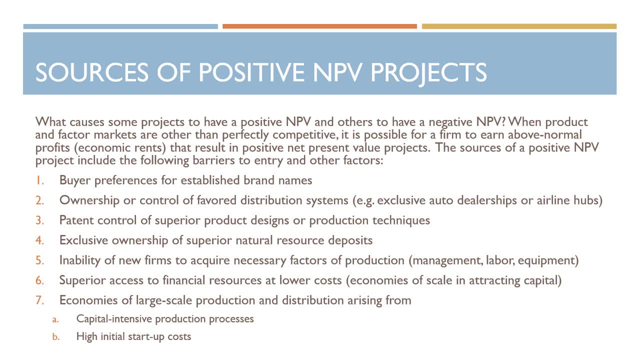 Uh, those are. those are the uh um, uh particular uh barriers that keep Competitive uh firms entering the same markets, um, so that uh the firm will have a better positions in the markets to fight for their profits. 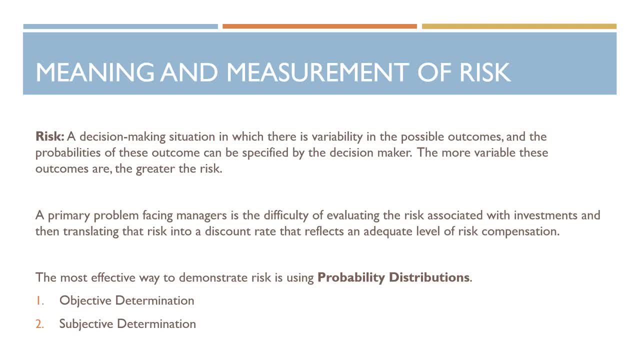 Now we talk about um how the marginal analysis is being uh considered um in economics and also how um we defined um uh those uh net present values um in returns Uh risk. 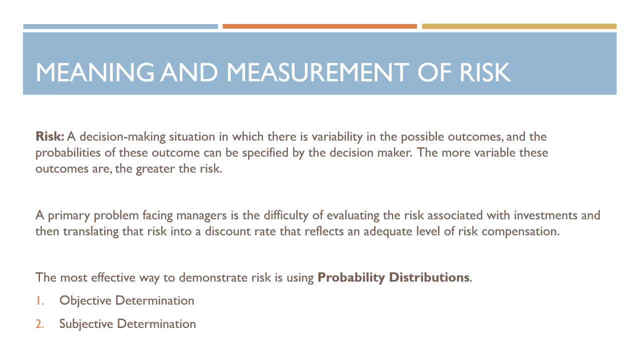 It's basically another big topic in um managerial economics Particularly, we we think about risks, uh that associate with almost everything that we are, we we make in decisions. Um one particular things that you can um imagine is that, um, when you have um five different projects um in front of you, um, each of this project might involve different returns and each of this project might also associate with a particular 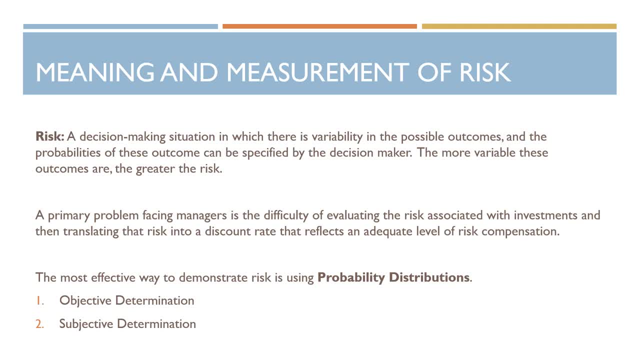 Types of risks. um taking an example like a construction projects, you might actually face the risk of um rising uh material prices, uh increase of labor costs or maybe sometimes postponed uh uh um uh projects by the government, uh uh licensings. 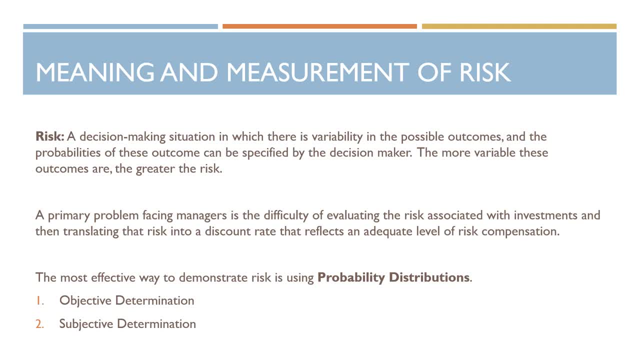 Um. so all of this are basically risks to take when the business take on the projects Um and other types of risks that you can imagine is to develop a new Software products that involve a lot of uh human capitals, um, software engineer, computer scientists- all this uh uh human resources uh pull into the products. uh that might uh post a very high uh initial cost of the company that they might not even be able to retrieve. uh those causes uh after the product uh or the service is launched. 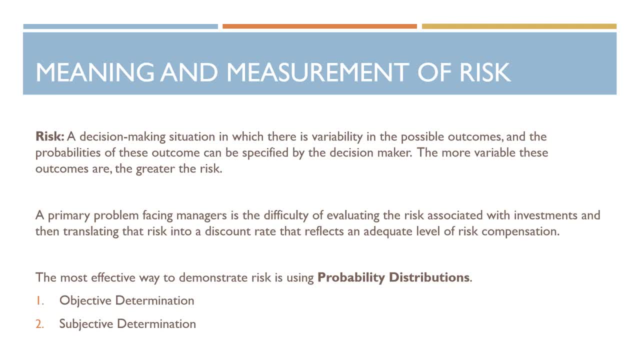 So every decisions, every projects, every uh operations Has different types of causes, Um, the most effective ways to determine uh or demonstrate risk. It's basically using a probability distribution approach that you can kind of take into account of the historical cases and, and look at it, most uh uh objectively. 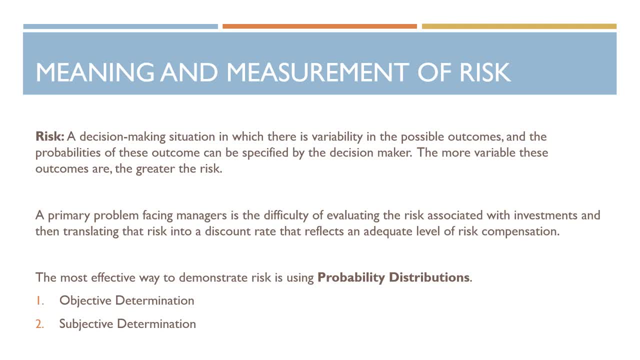 Um, so that you can determine whether the risks are um high or low comparing to the other related projects or uh uh, uh, uh, uh uh uh methods. So, generally speaking, managerial decisions can be made based on two. 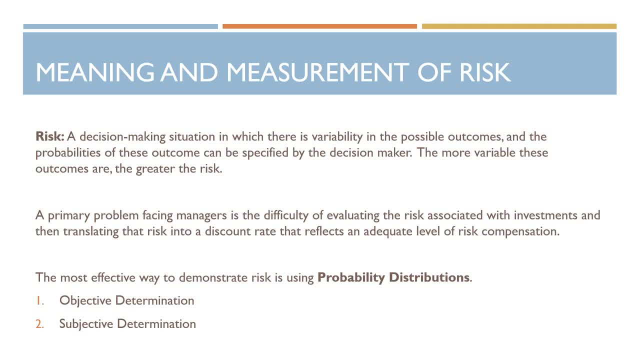 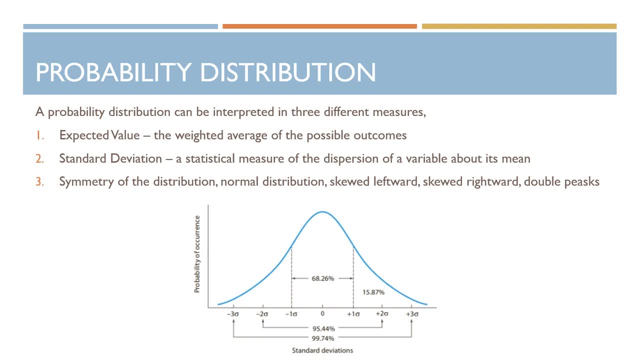 particular determinations, like objective determinations or subjective. So the objective approach, just like how I described it earlier, you can look at the expected returns of a project or maybe the expected cost of operations and look at the historical data and form a distribution to see: well, oh, 10 out of. 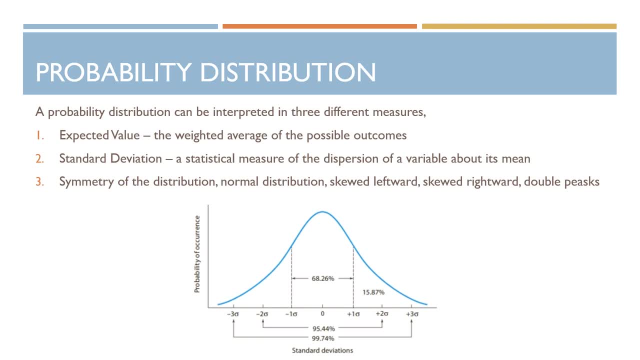 the 20 projects will have a loss and 5 of the same kind of projects out of the 20 will have net and then 5 out of the 20 will have a positive returns. In this case it's easy to see that the chance of success in this particular types of 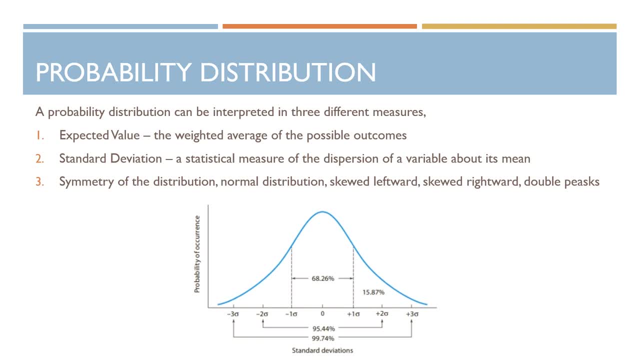 projects will be somehow relatively low versus if you have a investment projects that usually returns like 3 to 5% most of the time, where sometime this similar kinds of investment project might have a loss. but it's it's. it's a very, very short tail, like 1% of a. 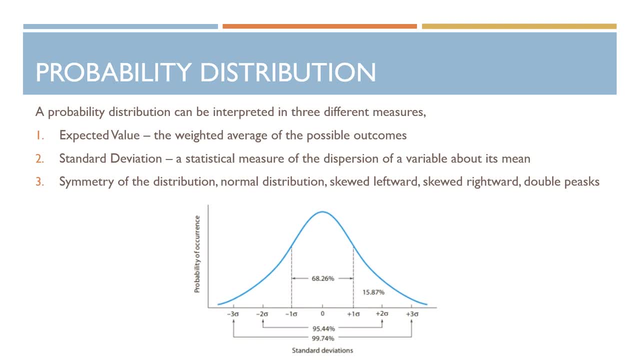 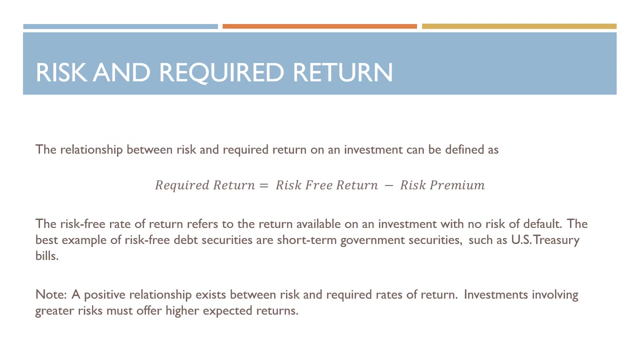 chance, but majority of the time they will earn high incomes returns. Then you will be able to tell the distribution has a lower risk on this kind of a risk to lose money. So the general idea is basically apply a statistical approach to evaluate the risk of a decisions in the business And, of course, 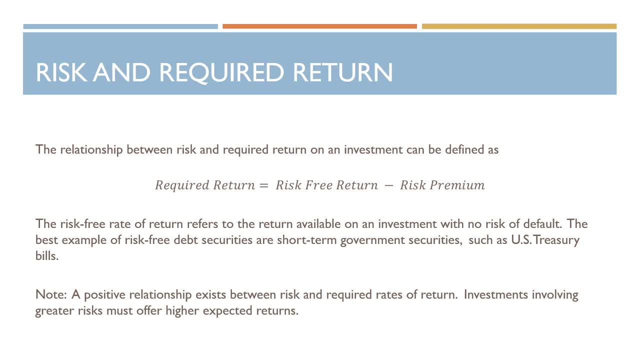 combining all this different analysis, or maybe future present values, calculations and risk determinations. we are basically focusing on just one thing, right? so what could be the potential returns if I'm gonna make that decision today for the company? And it all nails down to this: simple relationships, where the 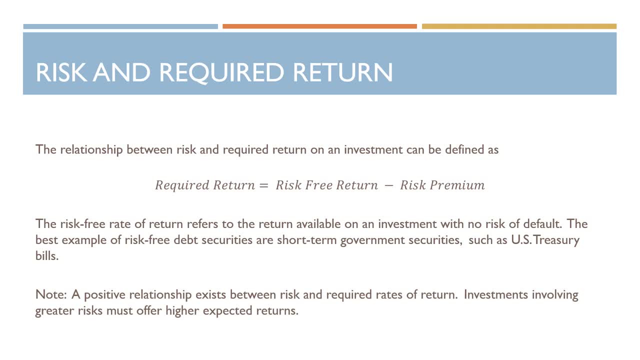 required return of a projects. it's literally just a risk-free returns minus the risk premium And what we define as a risk-free return. it's basically any returns from your investments or your resources that has no risk that can be post for the business. One easy way to think about a. 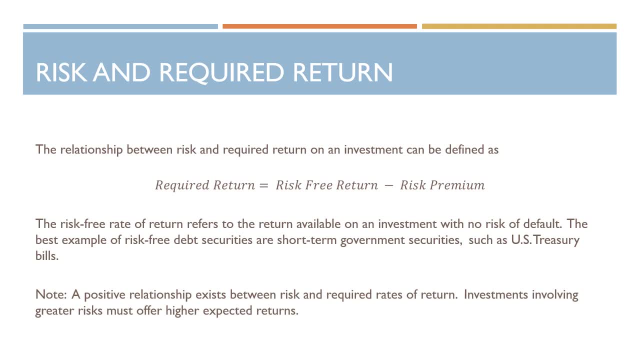 risk-free returns is to relate what you can do with your capital nowadays. For instance, an easy way to think about risk-free return it's using the US Treasury bill's interest rate to think about the returns in the future. For example, if the US Treasury bill overview a 3% for a short-term or maybe medium terms. 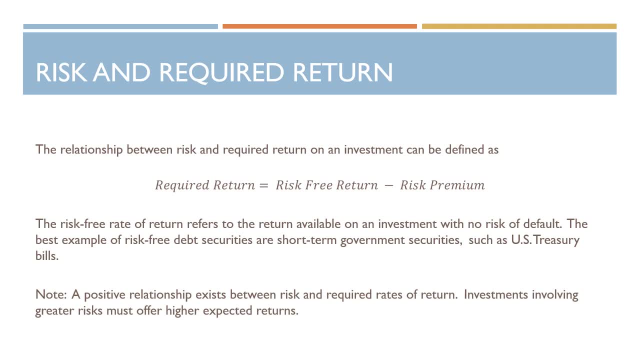 government security, 3% or 5% returns and- and you know, by the fact that the US government is going to pay you the money back after the security is matured, And that's a guaranteed returns, and that's basically what we call a. 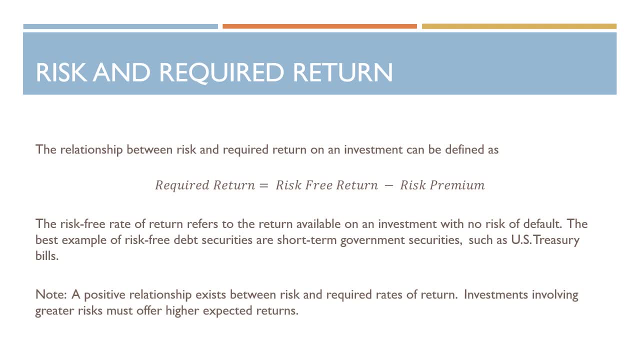 risk-free returns from your investments. On the other hand, you might also want to think about what are the risk premium factors here. So the risk premium factor is basically the risk that we talked about. So every single project has a particular types of risk: to lose money, or maybe net, or maybe earn.